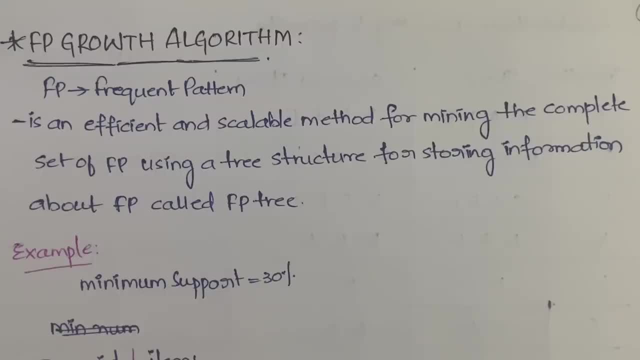 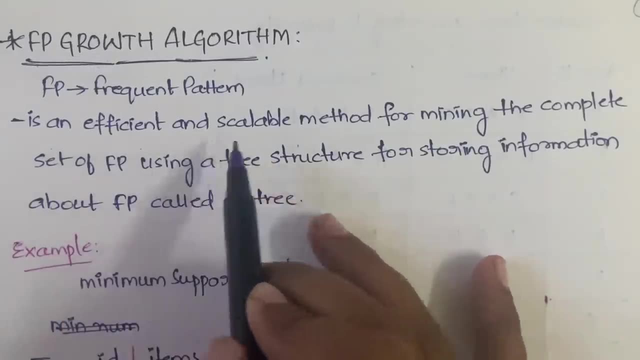 the end, and let's get into the video Now. first of all, what do you mean by FP growth? FP is nothing but frequent pattern, frequent pattern growth algorithm. Okay, it is an efficient and scalable method for mining the complete set of frequent patterns using a tree structure. 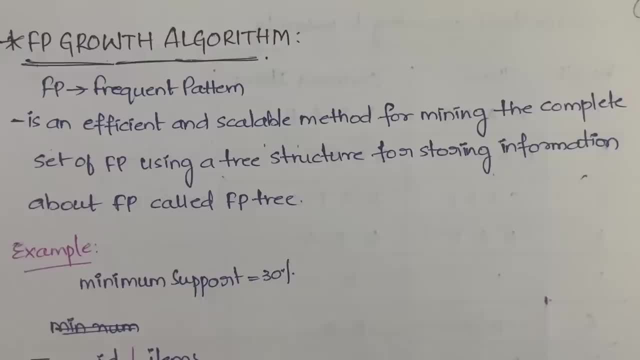 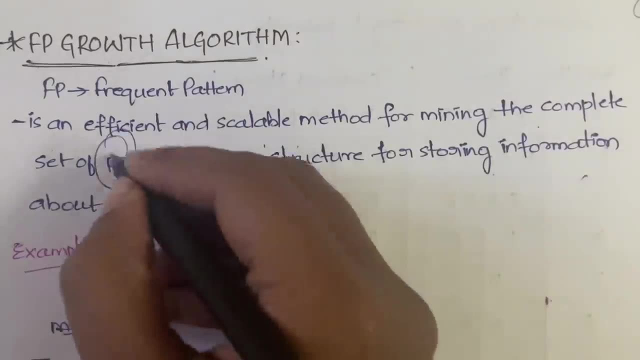 for storing the information about the frequent pattern, which is called as the FP tree, which means that it is a FP. It is an efficient and scalable method for mining the frequent patterns which are present- Whatever frequent patterns are present in the data- in order to mine those frequent. 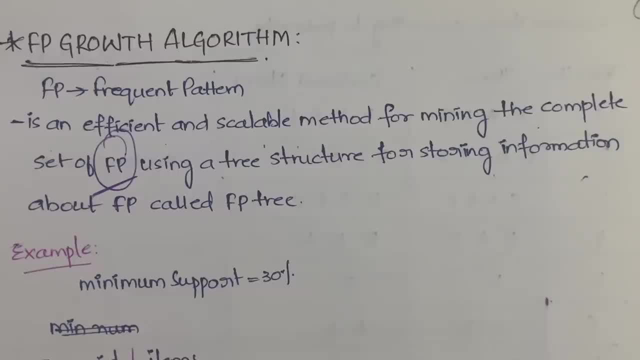 patterns. this FP growth will help you. This FP growth algorithm will help you. How this algorithm will work. It will use a tree structure. in form of a tree structure, it will give you the frequent patterns. Got it So for storing the information about the frequent. 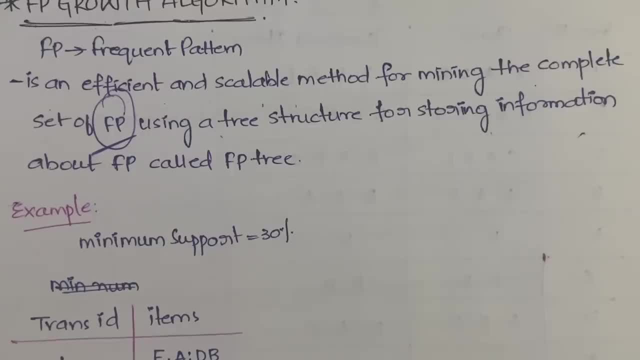 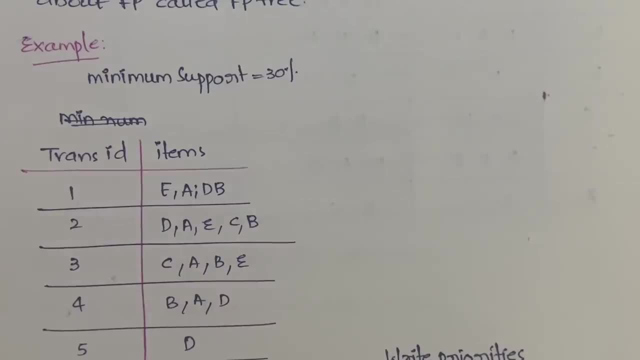 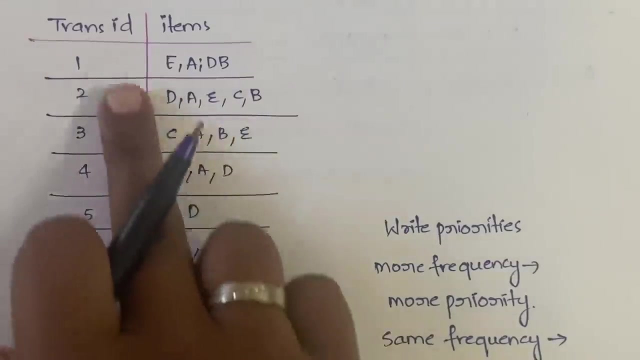 patterns, right. So this is about the FP growth. Now, for example, in the example, we have taken minimum support as 30%, Okay, and we have the- you know the example as this: one EADB to this is that we have eight transactions. 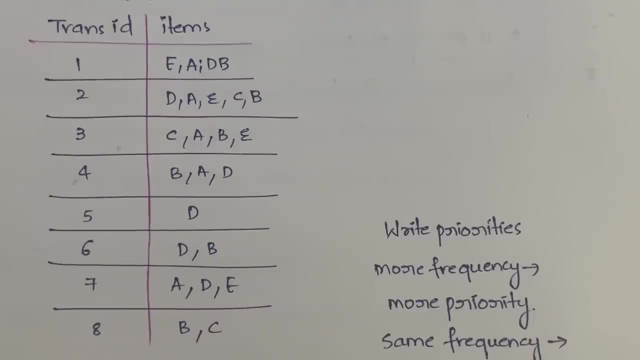 and we have items. Now what we have to do? same like a priori algorithm, only first we have to list out the individual items And for individual item we have to find out the frequency, okay, and then give the priorities. how to give the priorities, I'll tell you. 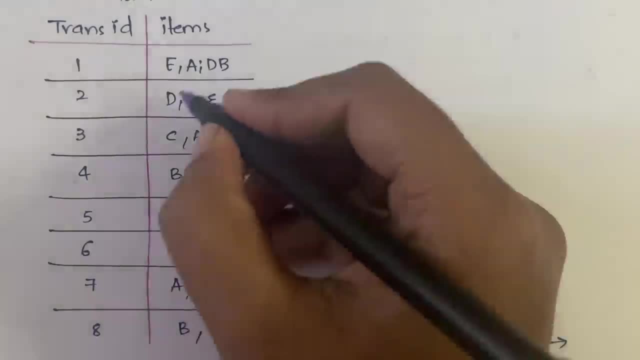 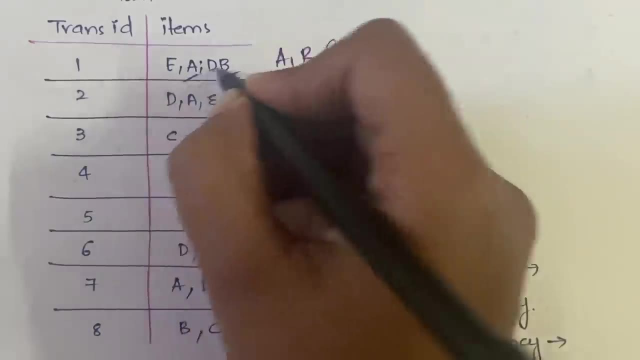 later. First step is to list out the individual items. So what are the individual items that you can get out of it? A, B and we have C- yes, C- and D and E. So these are the only individual items. you don't have F and any other thing, right? So you have. 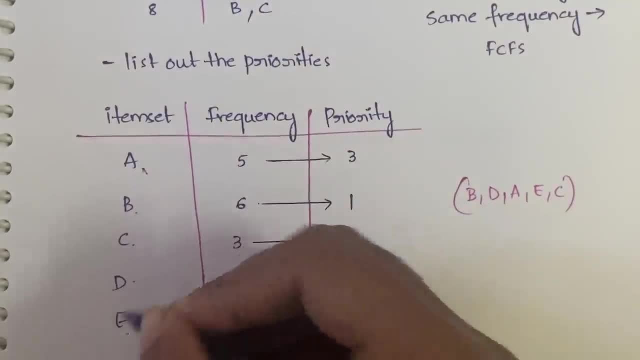 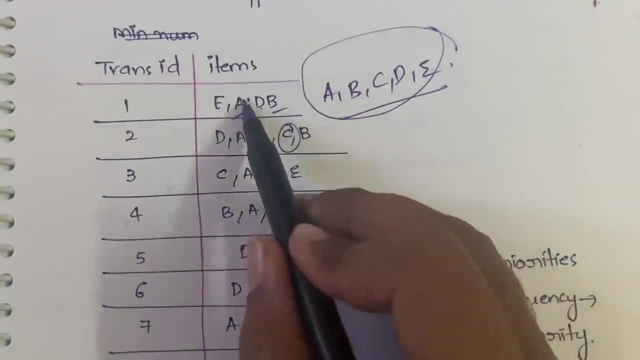 to first list out all those things: A, B, C, D, E. Okay, after you list out the individual items, you need to calculate the frequency. what is the frequency of A, 1,, 2,, 3,, 4,, 5,? frequency of A is 5.. And what is the frequency of B? 1,, 2,, 3,, 4,, 5,, 5,, 5,, 5,, 6,, 6,, 7,, 8,, 9,. 10,, 11,, 12,, 13,, 14,, 14,, 15,, 16,, 17,, 18,, 19, 20.. And what is the frequency of B 1,, 2,, 3,? 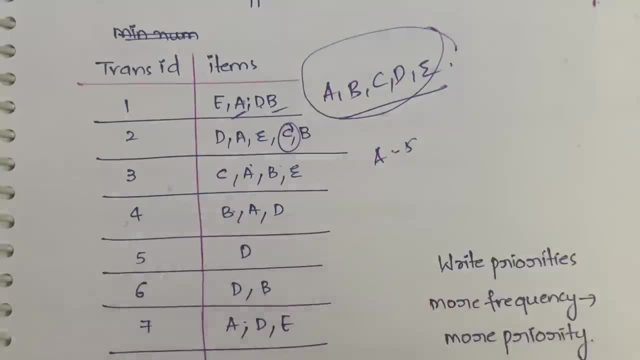 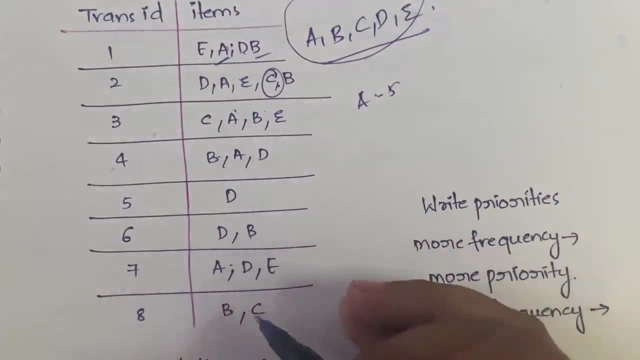 4,, 5,, 6, okay. Next, frequency of B is 6,. that is what we have written. Next, frequency of C: 1,, 2,, 3.. So frequency of C is 3.. Like that, you have to write the frequency of all the. 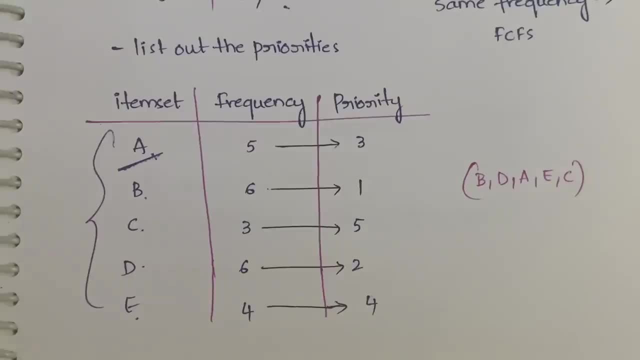 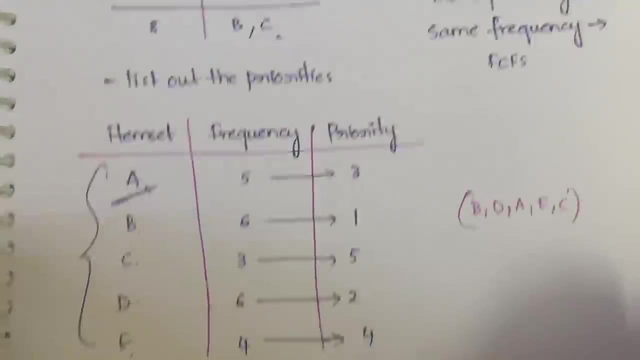 5 alphabets. okay, that is, 5 data set or items in the item set. After you write the frequency, you have to give the priorities. How you will give the priorities means Which is what, Which is having more frequency, that has to be given more priority And if any, two items. 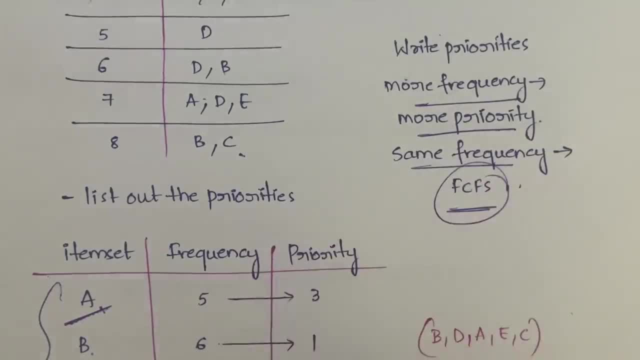 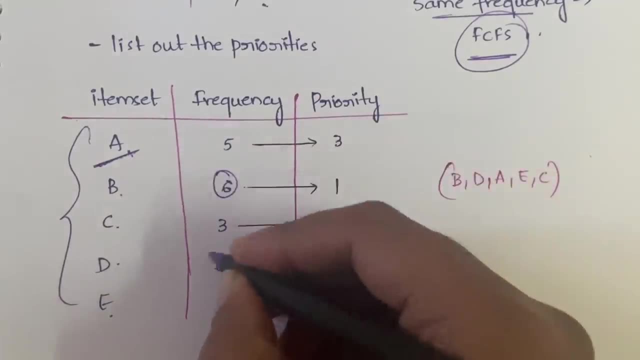 are having same frequency, which is first come, first serve basis. you have to give the priority, okay. So see here what is the highest priority: We have 6.. So 6 is for two items, right. So that is why first come, first serve, which is the first B. So B will be given 1. 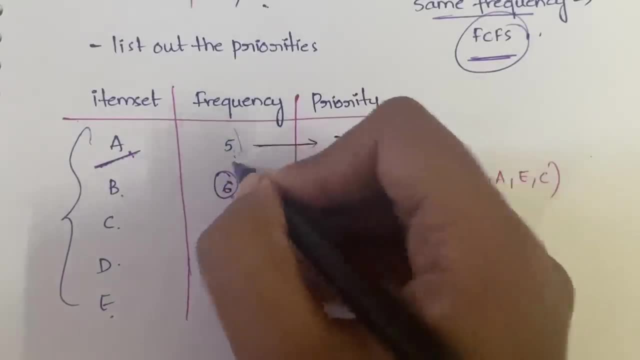 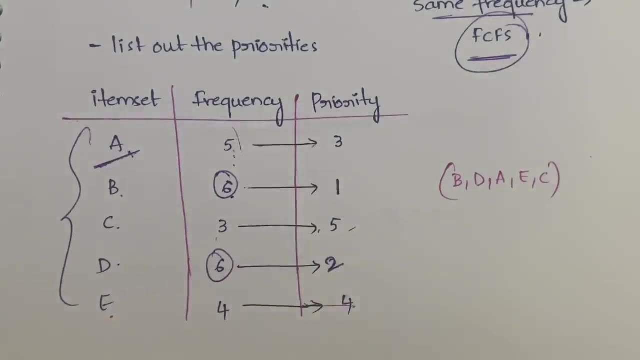 and next 2,, next 5.. 5 is only A alone has 5, so directly 3, directly 4 and directly 5, okay, Like that, you will be giving the priorities as well. Okay, so, in the order of priority, this is 1,, 2, 3, 4, 5, that is B, D, A, E, C, That 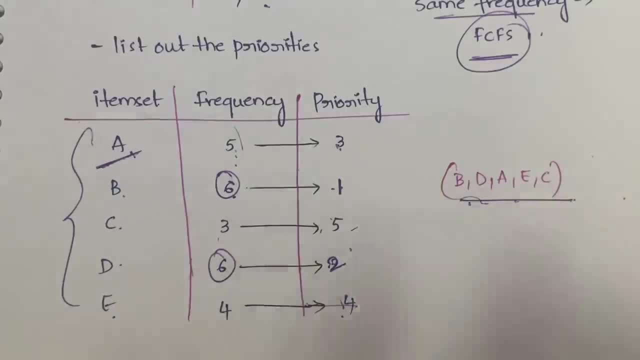 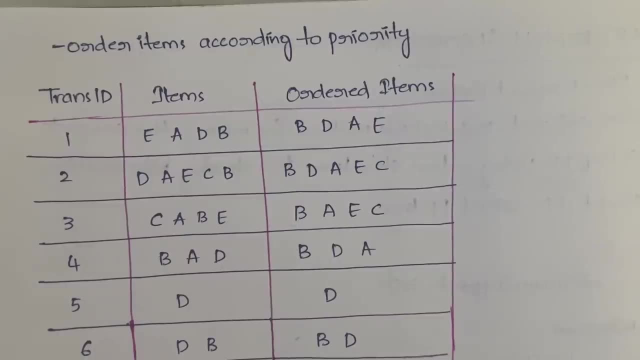 is what I have written here: B, D, A, E, C In the priorities, the priority order. you have to write it. Next step is you have to order the elements according to their priority, which means actually in the question. we have this right. We have the transaction ID and 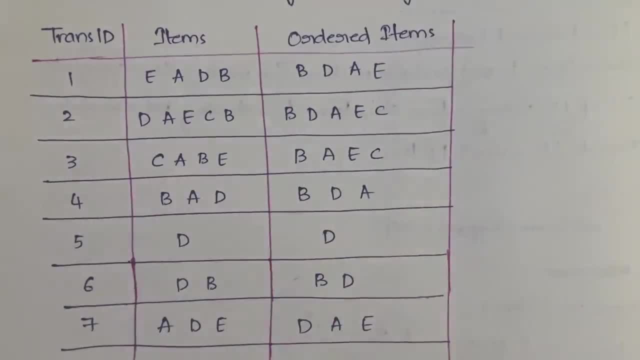 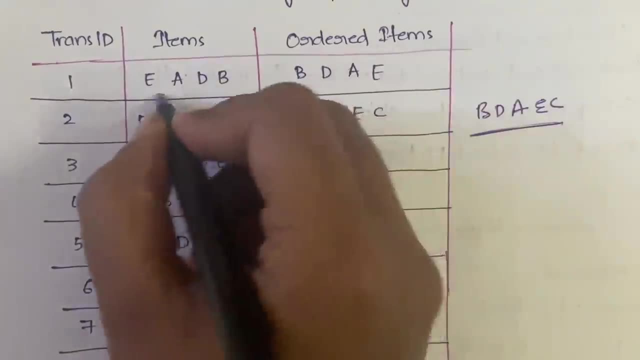 we have the items. So what is our priority? that we have got B, D, A, E, C. So according to this order we need to reorder these items which are given in the question. So according to the priority which comes first: B. So first is B next. 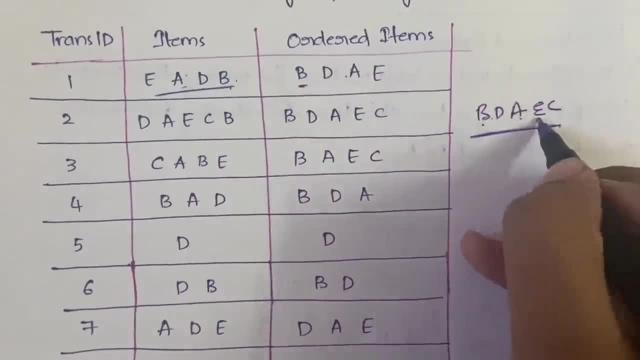 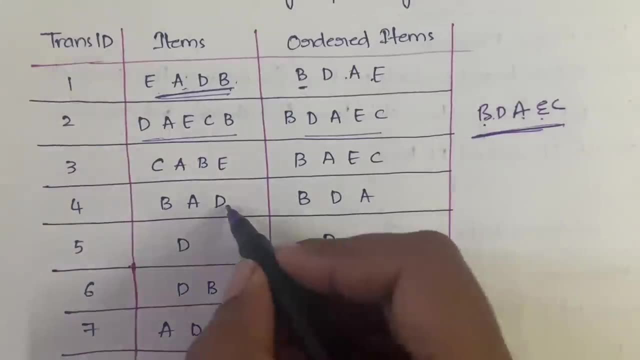 D, D, next A, A, next E, E, And we don't have C here, right, We can leave it, And this also should be ordered in the same way according to this. So, for example, you see this fourth. 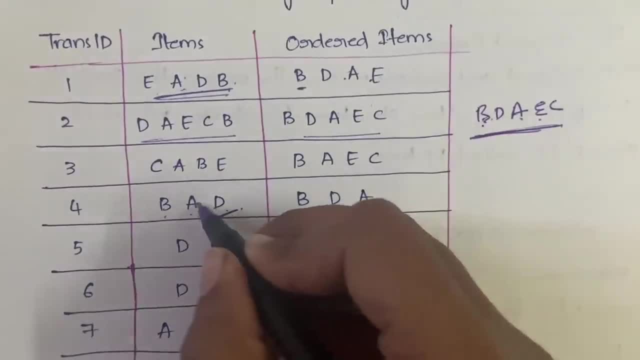 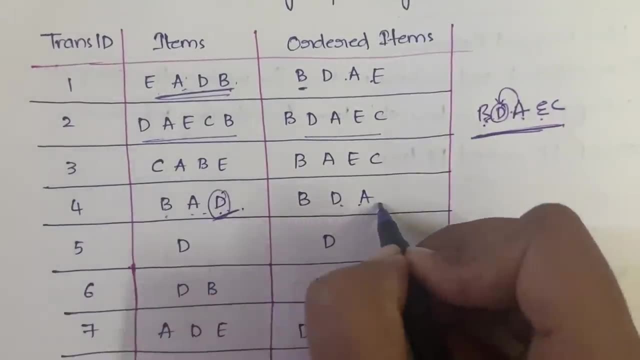 one it has. it is having B A D right. So first B, next A. But what is there before A? D is there? Do we have D here? Yes, we have. So B, D, A, it becomes Okay, So like. 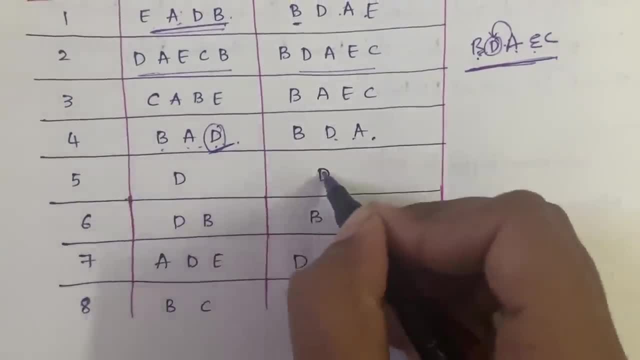 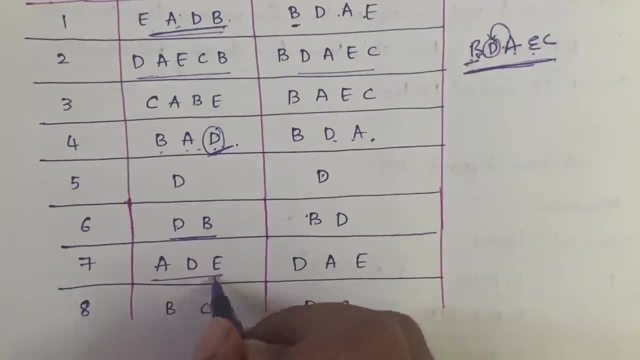 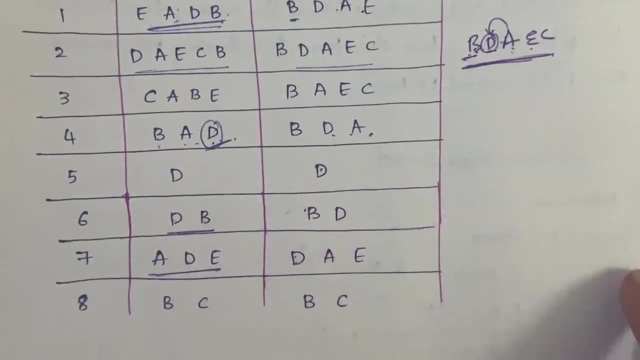 that you have to order everything in the priorities. D will be the same, D, B Among D and B, which is coming first here, B So B, later D. Next. we have A, D E here Among A, D E, which is coming first, D So D, Next after D, A E. Got it Like that you have. 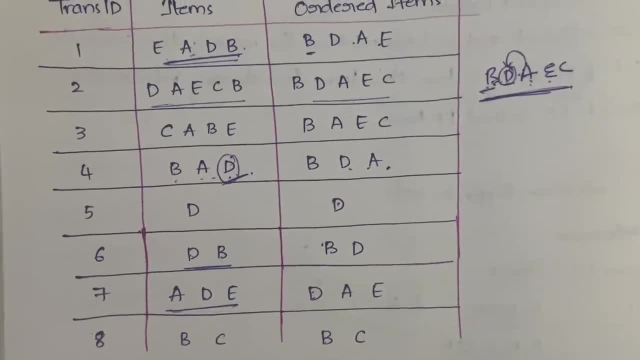 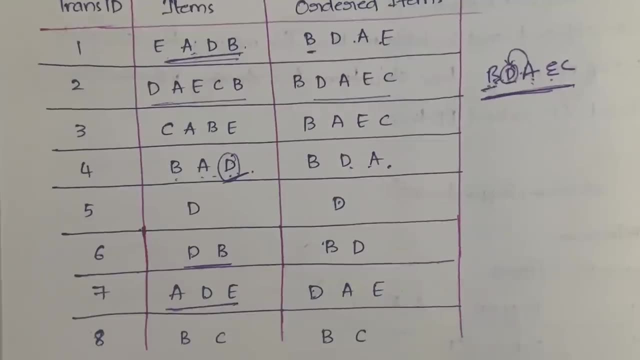 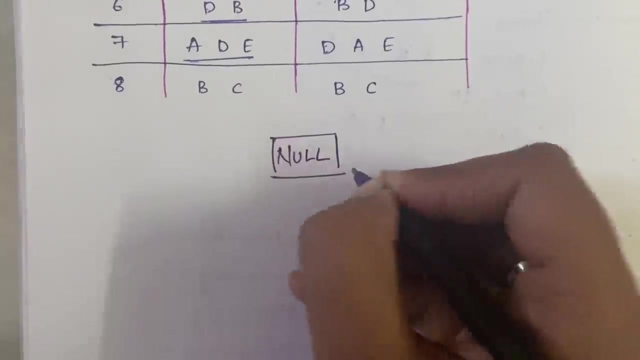 to order the items. you have to reorder the items according to their priorities. Now the task is to construct the tree. Okay, You have to construct the FP growth tree now, Okay, So for that, let us start constructing the tree. Initially, you will take it as null, Okay, Initially. 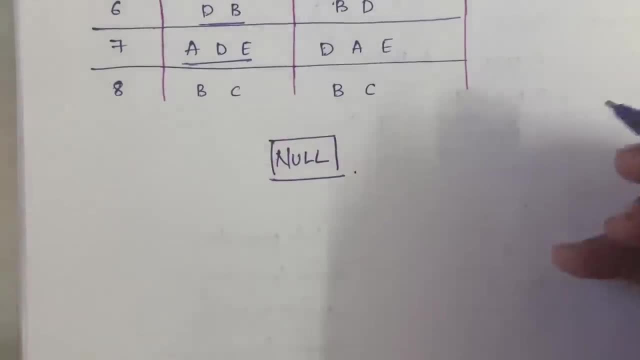 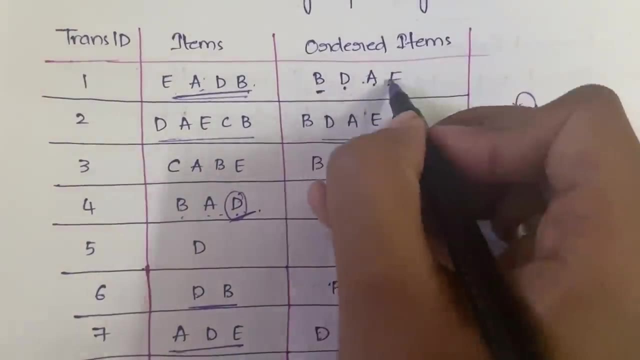 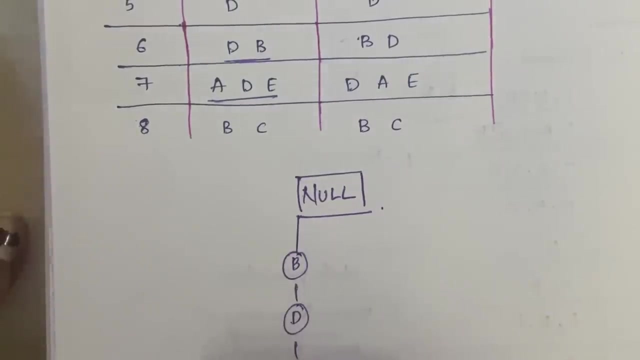 the root node will be null. Okay, Next, First, what is the in the first transaction, what is the first thing we are having? B D A E. right, So B D A E. Okay, So B D A. 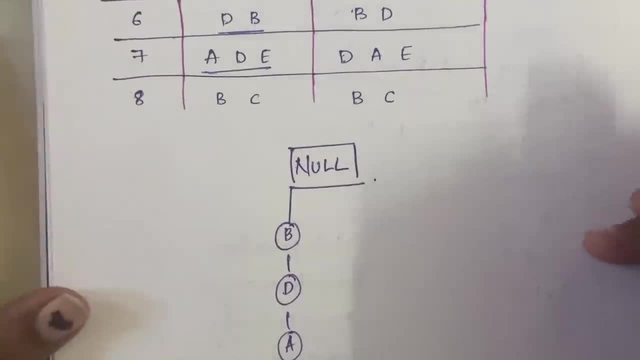 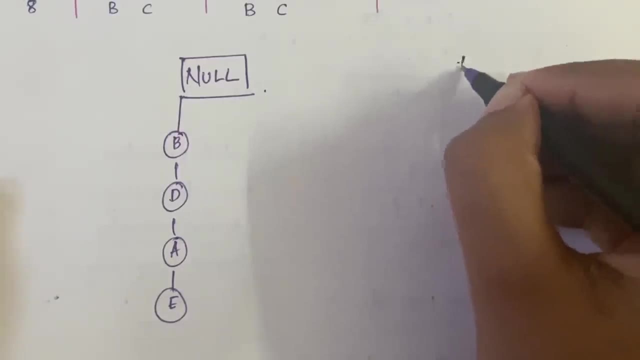 E. Like that. you have to construct the tree. Okay, B D A E. Correct. Here also let us write B D A E. I will tell you why. So 1, 1, 1, 1.. Because 1s. they have occurred All. 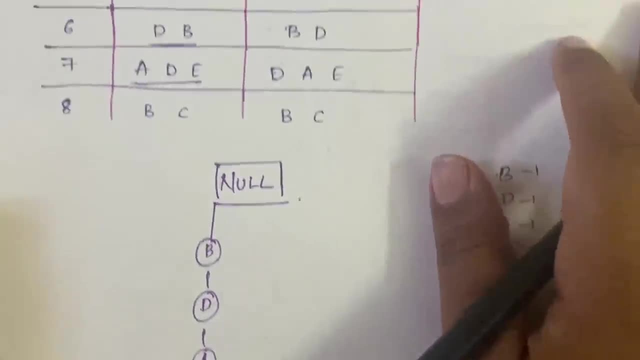 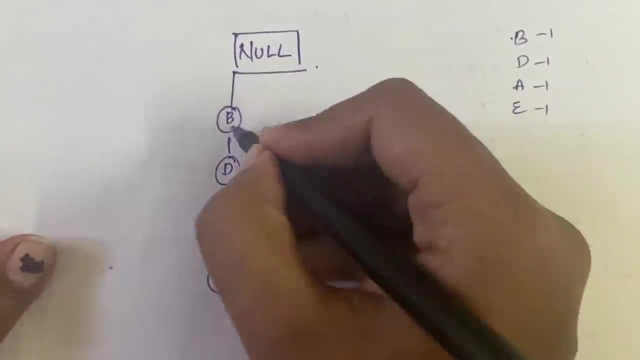 1, 1.. Like that, after writing, the occurrences go to the next one. Next sequence is: what do you want? You want B D, A, E, C. Right, So we have B D, A E, But we don't have. 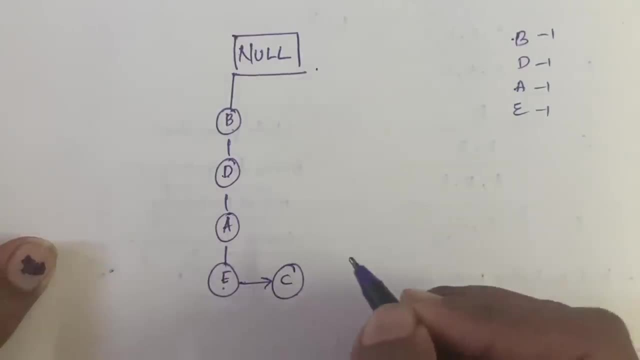 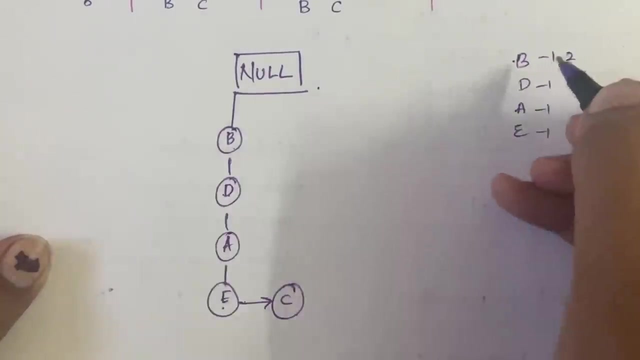 C, So write C. Got it Now. what are the occurrences? 1, 2. Because it is occurring for the second time In the second transaction. it has occurred Right Again. this also has occurred in the second transaction, A also has occurred, E also has occurred And C has occurred for. 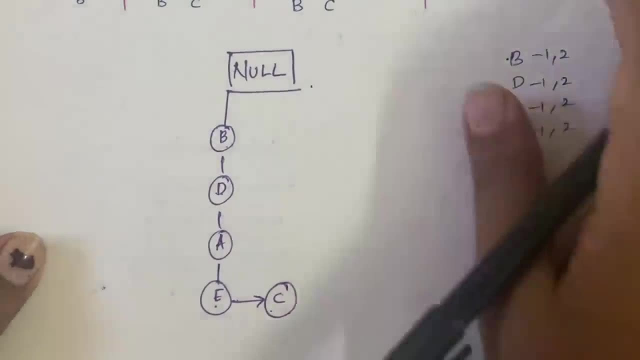 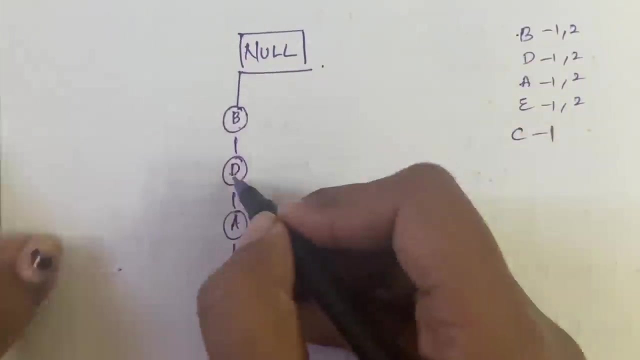 only one time, So we have written that Done. Next is B A E C. So for B. here we have attached What does that mean? B, D A E C- So for B. here we have attached What. 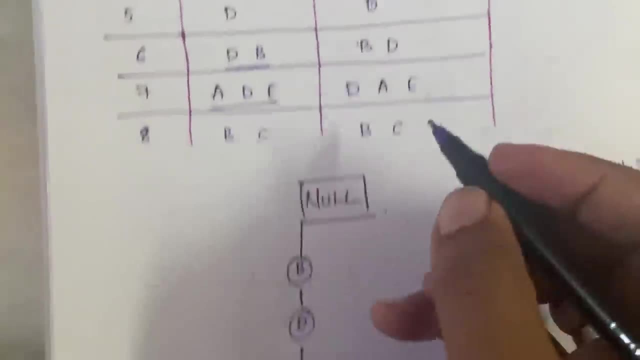 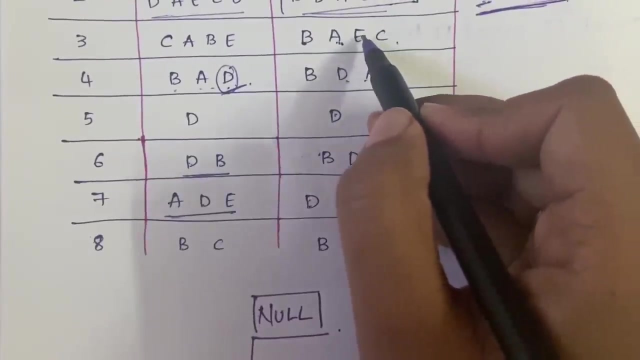 do we have attached D? But here we have A Right. So that is why we have to create a new node, now A And next E, C Right. So for A we need to attach E, And then we need. 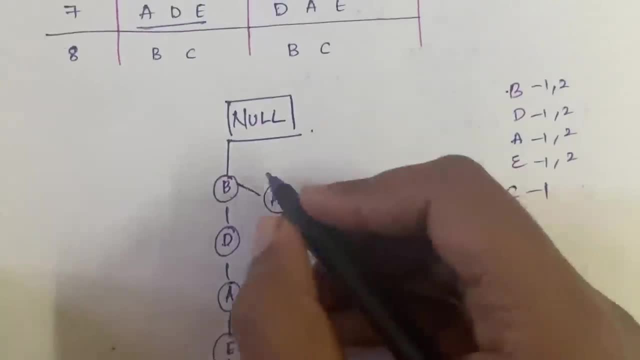 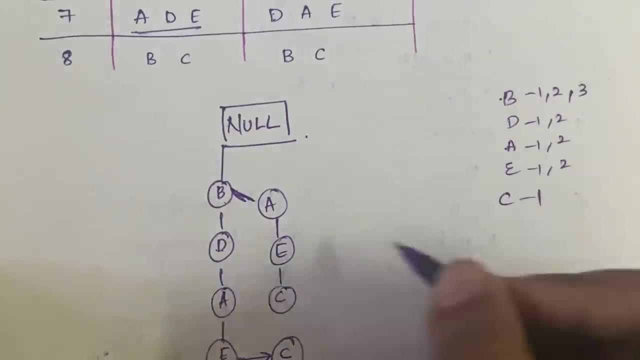 to attach C. Got it Now. the new transaction will become: So we have not started from the null Right, So we have started from B. So for B it becomes comma 3.. And next A, We have this. A is this one which is attached to D, So we don't update here. We will again. 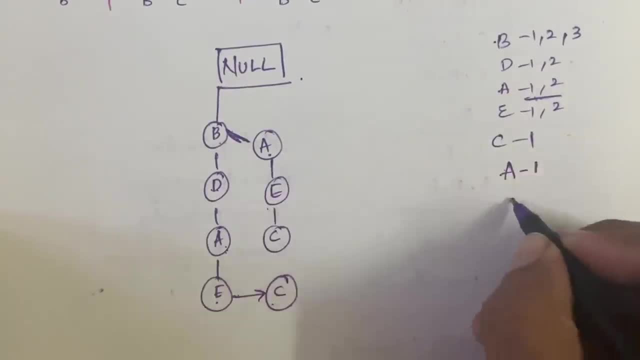 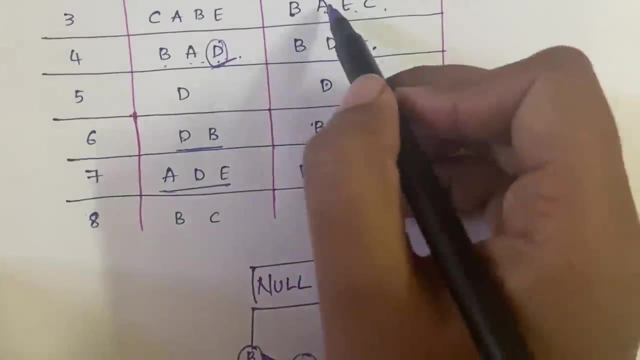 write A freshly, Write 1.. And E fresh again, 1. C fresh And 1. Got it. So now we are done with the B A E C as well. Next comes the B D A. The fourth transaction is B D A. 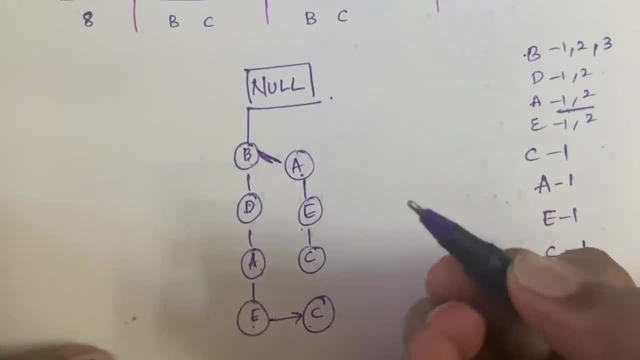 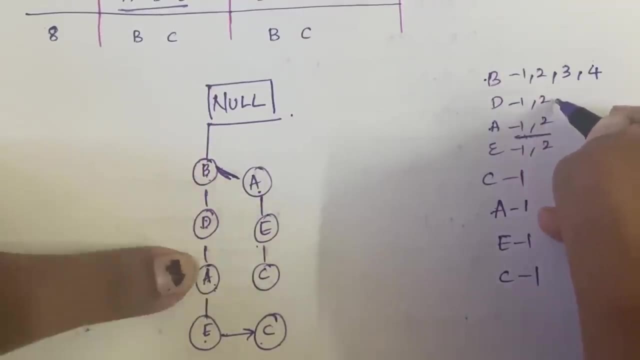 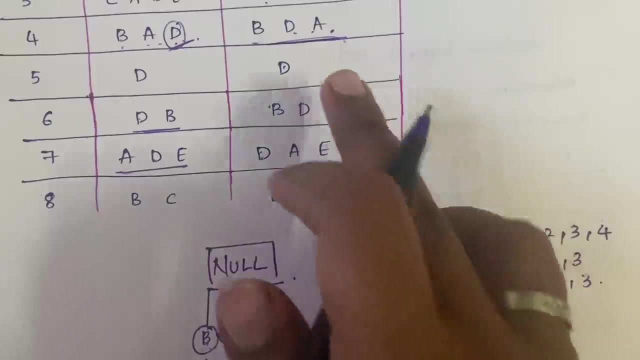 We have B, D, A already, So we need not write a new transaction. We have to just update the occurrences. So B, what is the last number? 3. Right Now it becomes 4. D A, Right, So 3 and 3. Got it. Next We have D, So separately, we don't have D for. 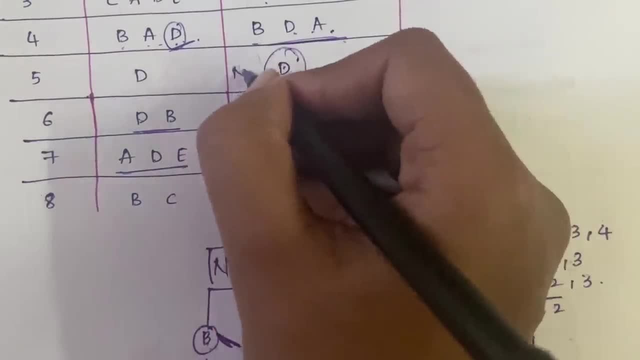 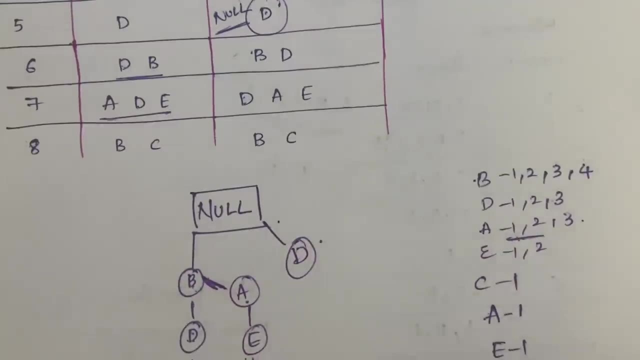 null. We have only D. Right Before D, we don't have anything, which means it is null. Okay, That is, you have to start the transaction from D, From null. So here D will come. Got it Now, for again, you will write a new transaction. here D is equal to 1.. Why you are not updating? 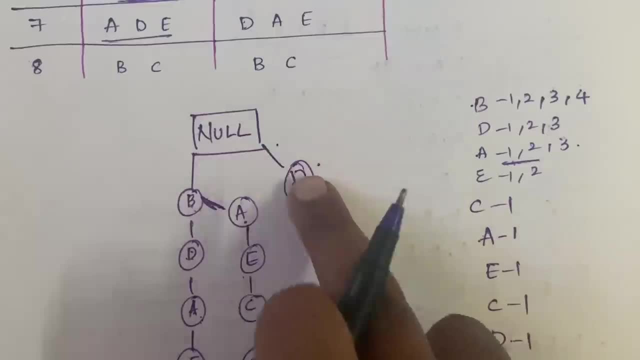 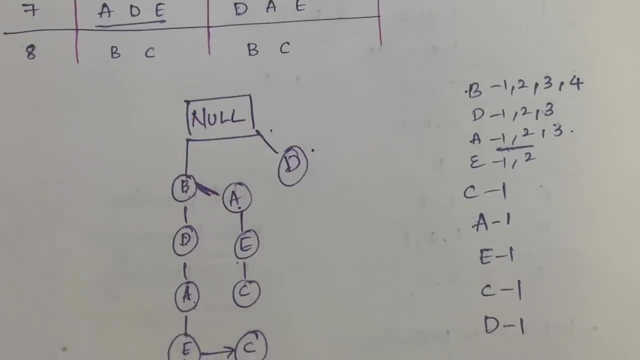 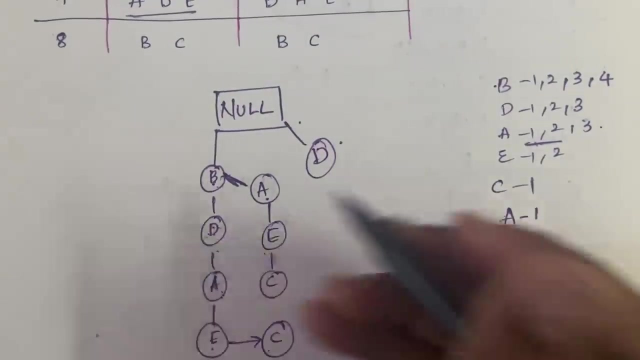 here. This D is related to this one which is attached to the B, Not the root node. Right, Got it. That is why you will not directly attach it Now. after that, next transaction is B D, So do we have B D? Yes, we have B D, B D, Got it, So you have to just update. 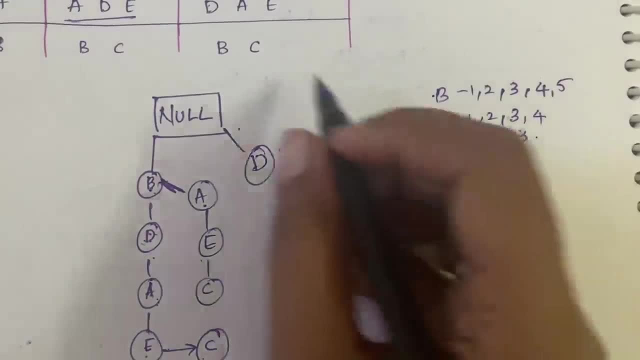 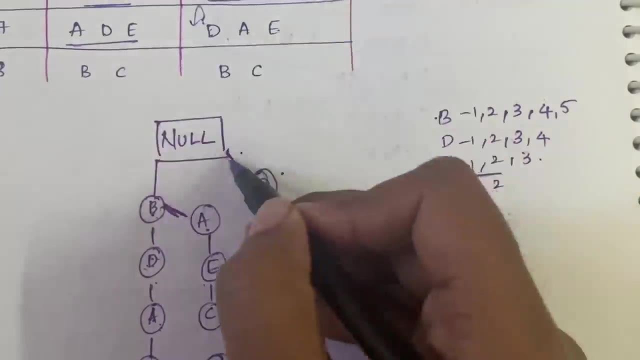 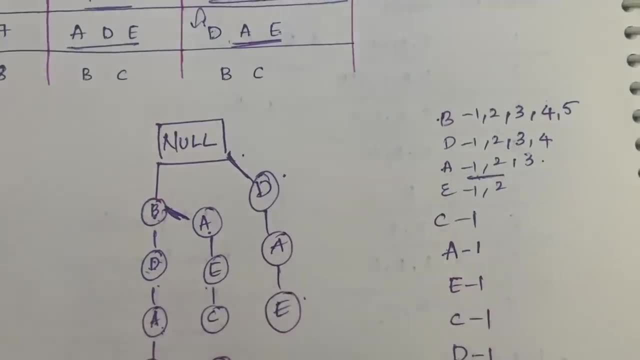 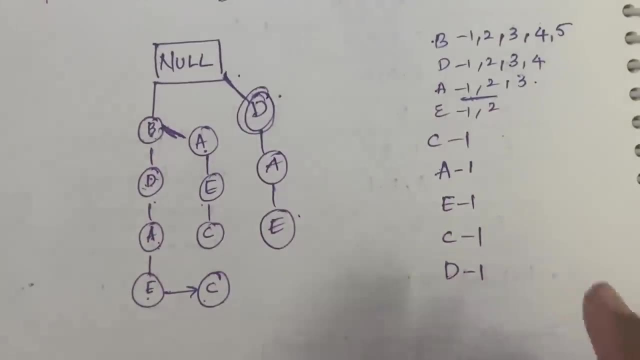 A, E. We are newly attaching Right, So now what you have to write, what is the for this D we have written here: D is equal to 1.. 1, 2, because we are using it for the second time. 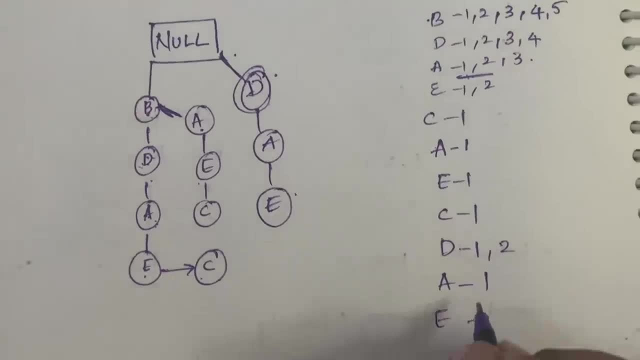 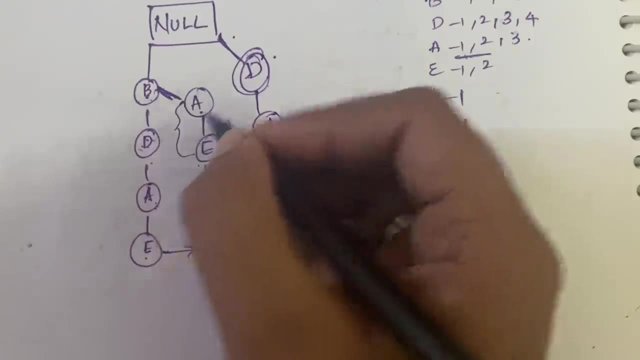 Next write A newly again and E newly again. Why newly? we are writing here Here. we have already written newly for one time, Right, But this is for this transaction. Got it For this transaction again, we have to write newly. So E is equal to 1.. You will get Now. 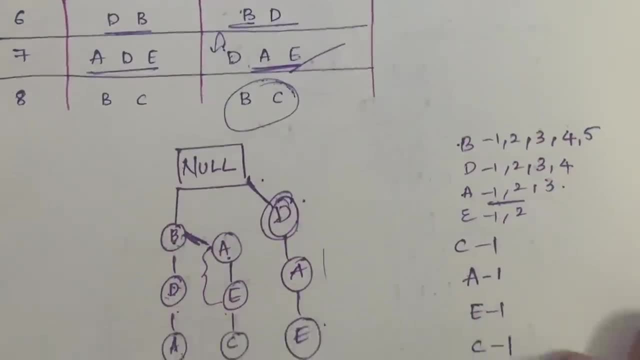 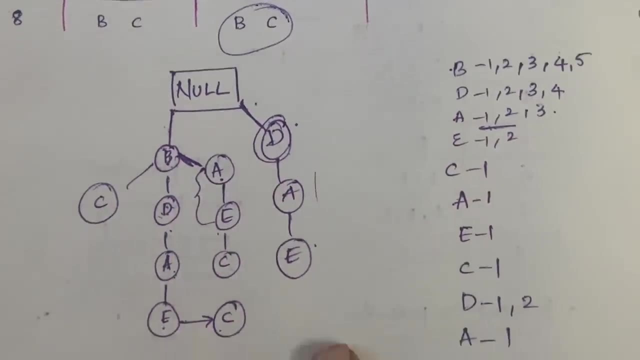 what we have done with D, A, E as well. The last is B, C, So B root for the null. we have B attached, So here you can write C, Okay. So again you have to update the occurrences. This B belongs to the first one, Right? So again you got a new transaction from it, since. 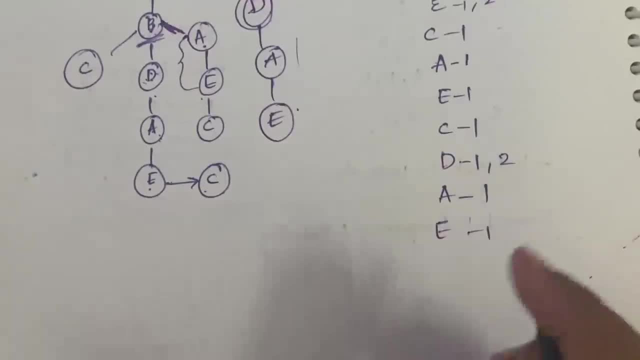 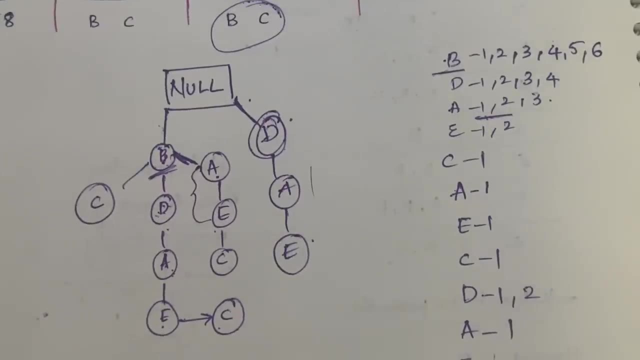 you have. write it as 6.. And C is a new one, So C is equal to 1.. You will write: Got it. So this is how you construct the tree: by using the transactions, By using the transactions which are in the order. 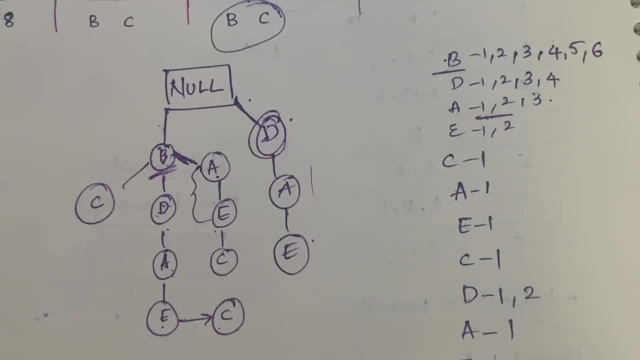 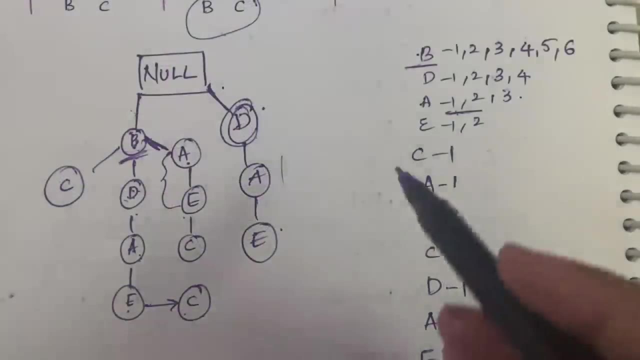 First what you have to do. You have to first list out the priorities. Then, according to the priorities, you have to rearrange the items given in the question and then construct the tree. Got it Now. why did we write this, then These occurrences? why did we write? I will 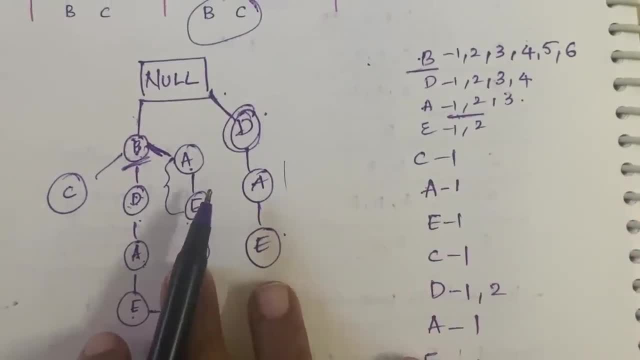 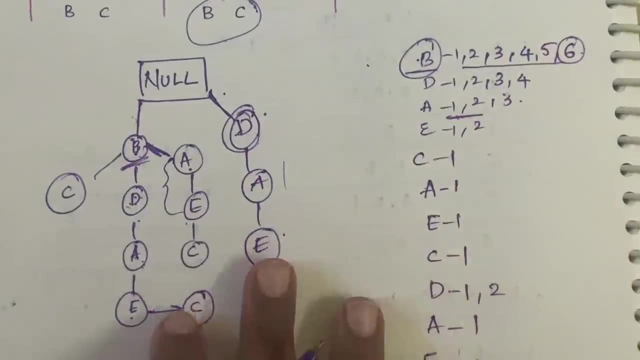 tell you. This is to check whether you got the answer correctly or not. How you will check, See here how many times we have B. Only one time, Right, Only one time, and how many occurrences 6.. So now you have to check the frequency of 6 in the question. Okay, 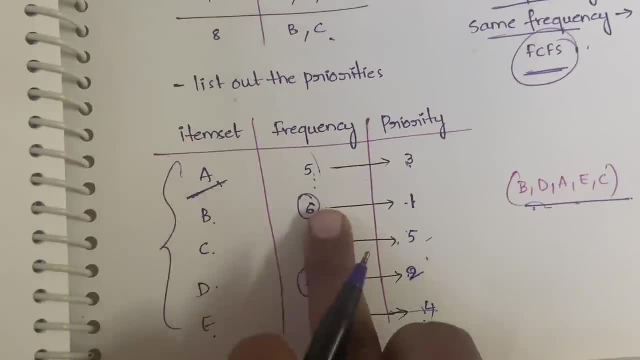 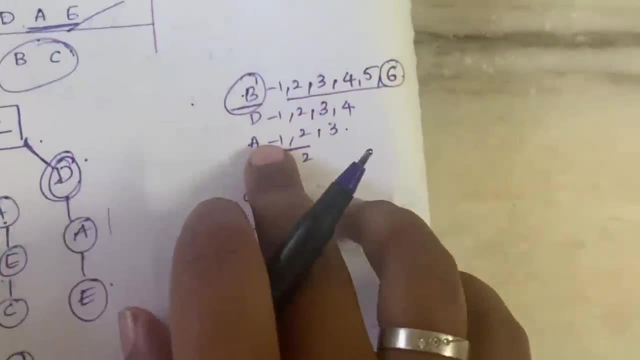 See, Sorry, B. What is the frequency of B? It is 6.. Got it. So 6, 6, same. So it is correct. Now let us check the same thing for D as well. So for D, 1,, 2,, 3,, 4 and anywhere else, Yes, Here. 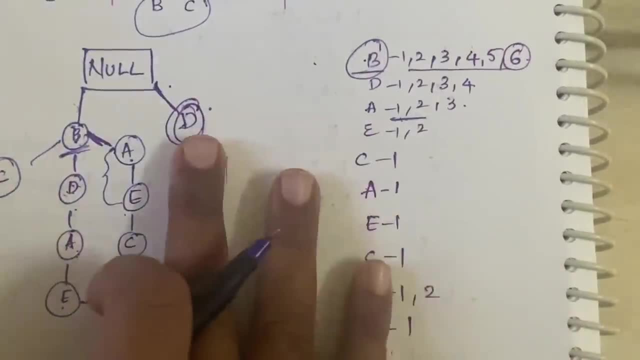 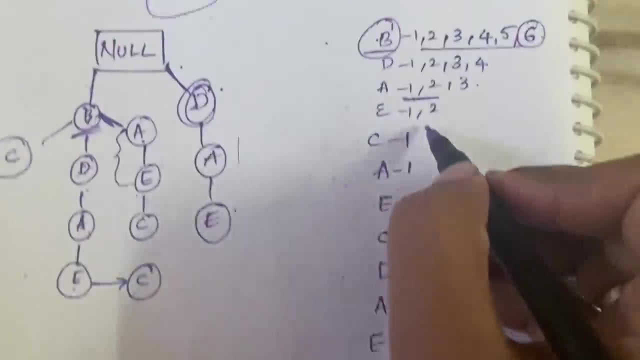 Again 5,, 6 and anywhere else No Right, So 6.. Let us check 6: is the priority of D, frequency of D or not? Correct 6.. Next, let us check for another one as well. A For A, we have 1,. 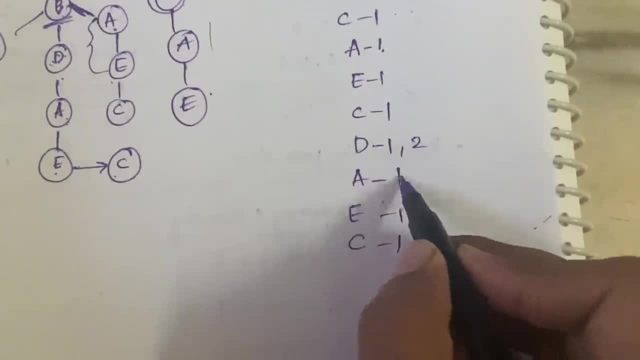 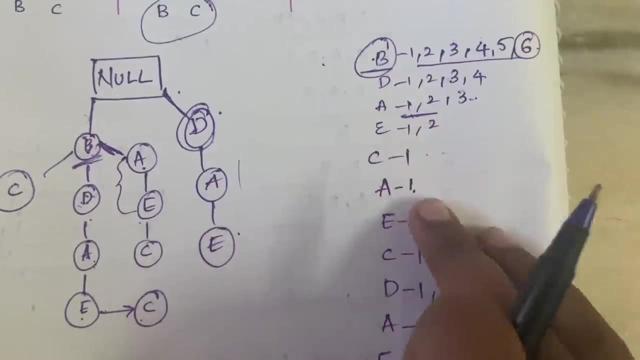 2, 3.. Again, 4,, 3,, 4.. Okay, And 5.. The frequency of A is 5.. Okay, For next we have E, And for E it is 1,, 2 and 3. 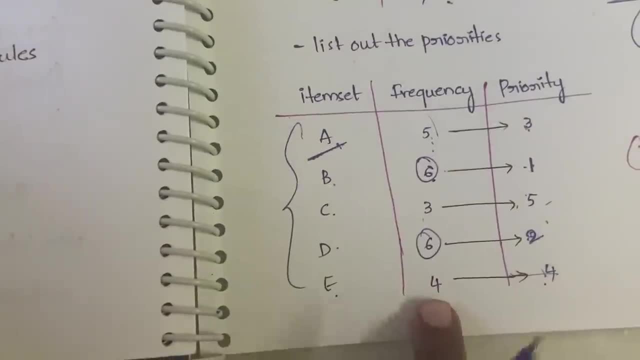 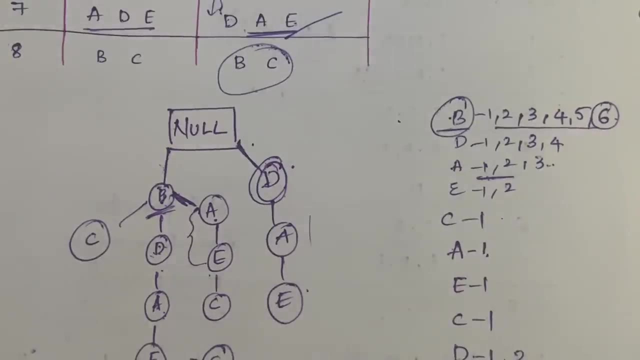 and 4. Here, Okay, So here it is 4.. Like that you can check whether whatever you got is correct or not. In that way you can check. So this count has to match with the frequency given in the question. Okay, This is about Fp growth. That's all I hope you understood. 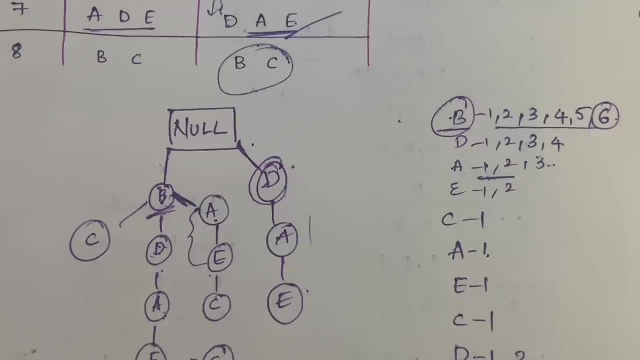 clearly what I explained. I tried my level best to make it very clear to you. Okay, So see you in the next class. Bye, So thanks for watching the video till the end And if you are still having any doubts, apart from what I have explained in this video, let me know in the comment section. I will.